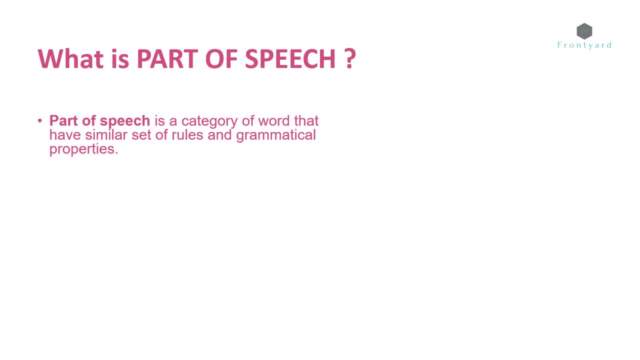 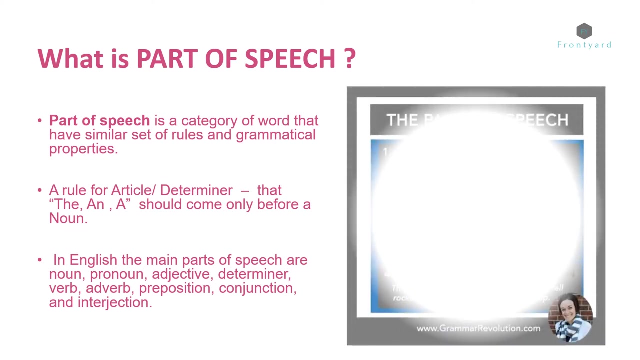 of speech is a category of word that have similar set of rules and grammatical properties. Example for a rule is for article or determiner, For the words the and a should come only before a noun In English. the main part of speech are noun pronoun adjective In English. 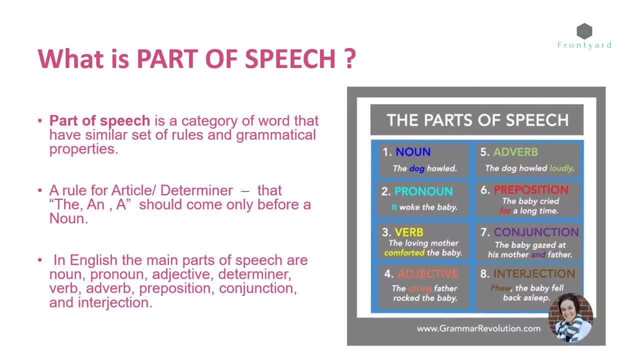 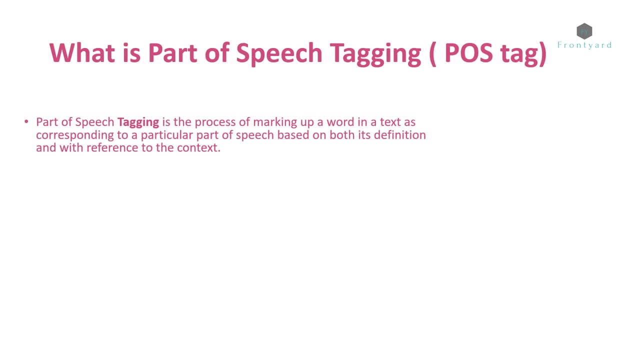 adjective, determiner, verb, adverb, preposition, conjunction and interjection. There are some more parts of speech, but they are not as commonly used as these are. What is POS? tagging Part of speech? tagging is the process of marking up a word in a text. 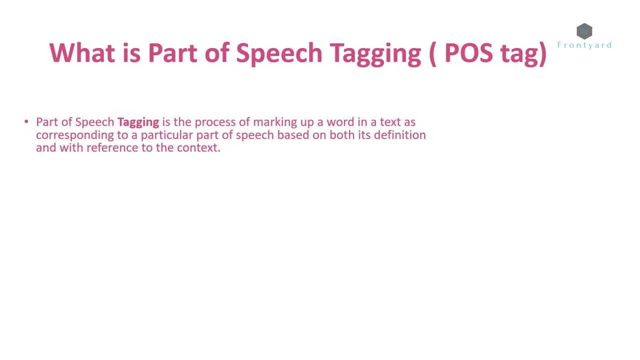 as corresponding to a particular part of speech, based on its definition and with reference to the context. Often, other grammatical words are used to mark up a word in a text. Other grammatical categories, such as tense, plural or singular case, are also included. 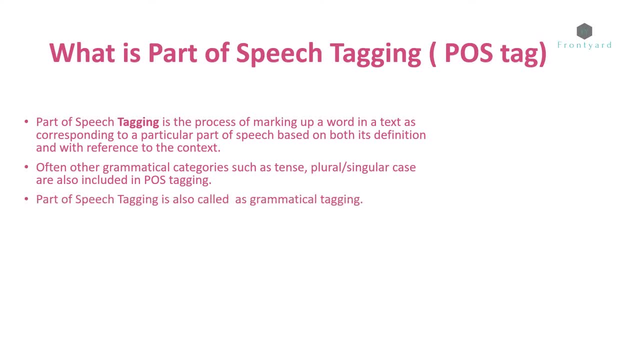 in POS tagging. The part of speech tagging is also called as grammatical tagging. Here is an example. The text says: I ended up watching the movie, So let us see how each word will be given a POS tag. The word I is given PRP, PRP. the first word, P, stands. 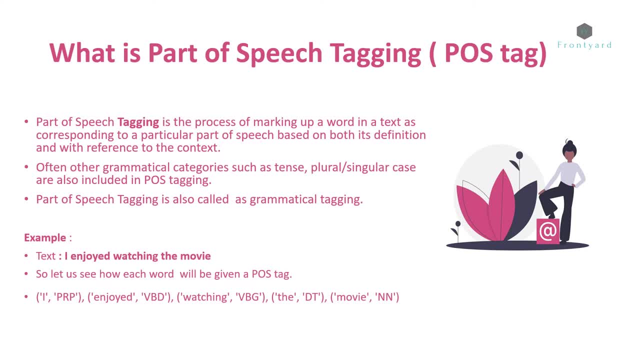 for pronoun Enjoyed and watching, has the terms VBD and VBG allocated, which means that the first word V stands for verb, For the, THE, the, it is a determiner and it is given D. NMovee is noun, So it is. 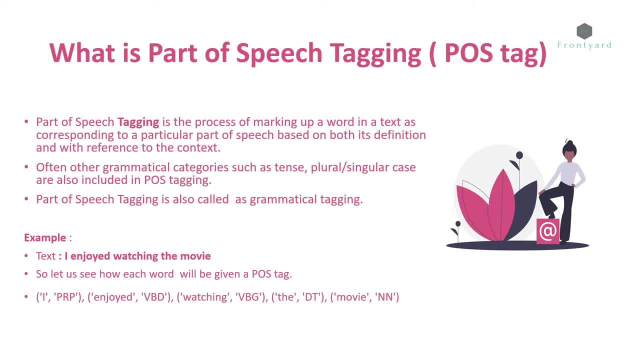 given as the first word NMovee In NLP, we will be able to identifier for each word what is the part of speech like noun, argument, pronoun Rome or determiner – as well. It is not very complicated to know. 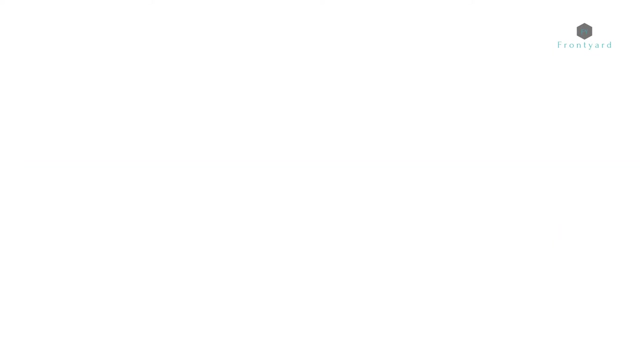 will be able to identify each part of speech. The part of speech tagging can be broadly classified into two types: rule-based POS tagging and stochastic-based POS tagging. Rule-based POS tagging: It uses a set of rules or algorithm to find out the part of speech. 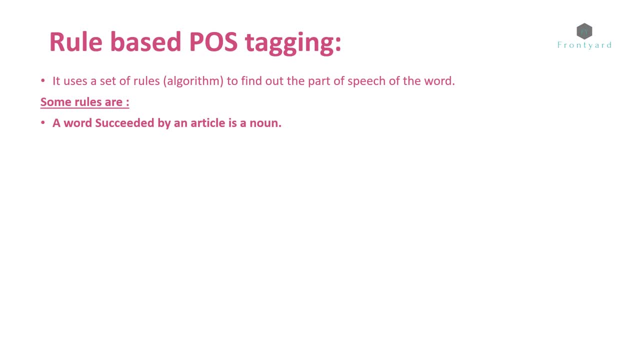 for a particular word. Some rules are: a word succeeded by an article is a noun. Here is a text that says that I saw a child going to the supermarket to buy an apple Here find out the noun. So the nouns are: child, supermarket, apple. So all the nouns are preceded by an article. So 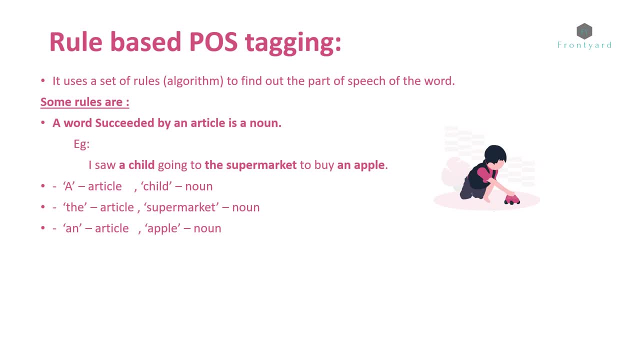 in the reverse we can say that if there is an article existing in the sentence, then the word succeeded by it is a noun. So in the reverse we can say that if there is an article existing in the sentence, then the word succeeded by it is definitely a noun. Here is an another rule A. 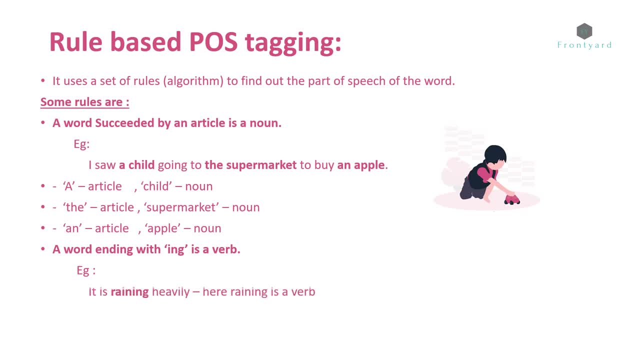 word ending with ing is a verb. Here is a text that says that it is raining heavily, So the word raining has ing. Here it is a verb. But if you look at the next sentence, it says that I enjoy the rain. Here the word rain is common for the previous sentence and this sentence, but adding: 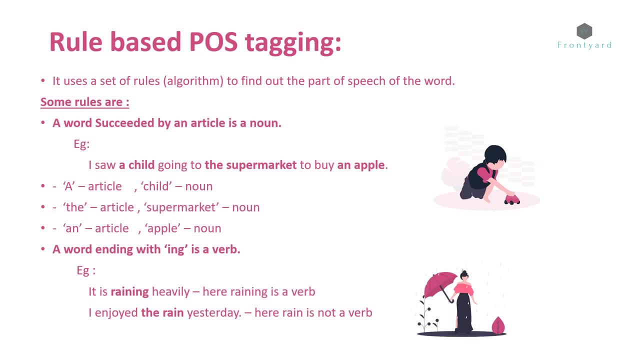 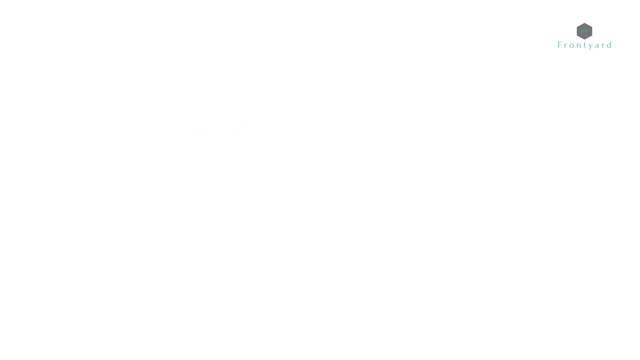 an ing makes it a verb If there is a word ending with ing as a gerund, so that words with ing can be definitely considered as a verb. 7. SOCASTIC-BASED TAGGING: Any model which incorporates frequency or probability of words in a paragraph or huge text to identify the part of speech are labeled. 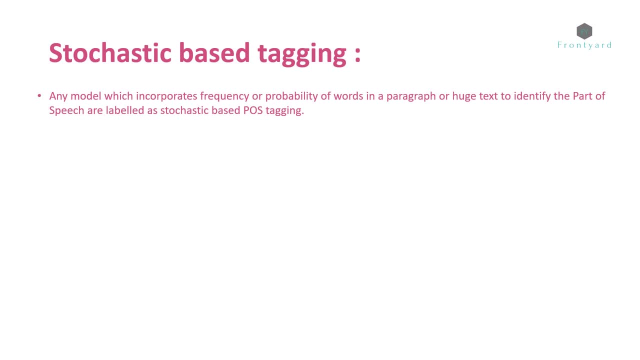 as SOCASTIC-BASED POS TAGGING. After a few minutes I will explain this with an example: io Under stochastic based tagging. there are many methods or models based on different approaches. Out of them, I will explain a model called tag sequence probabilities. 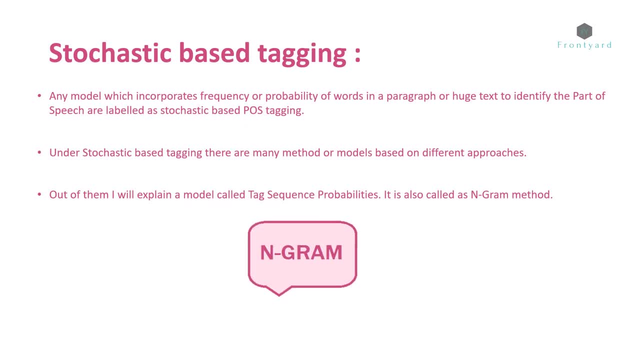 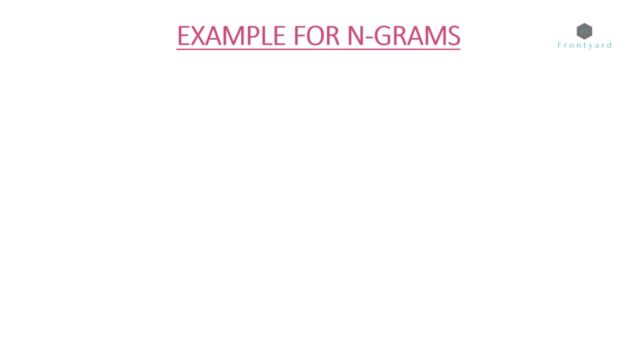 It is also called as N-gram methods. The N-gram is all about creating pair of words in N count from a sentence. With an example of N-gram, let us understand how stochastic based tagging works. Here is a text that says: I enjoyed the movie. 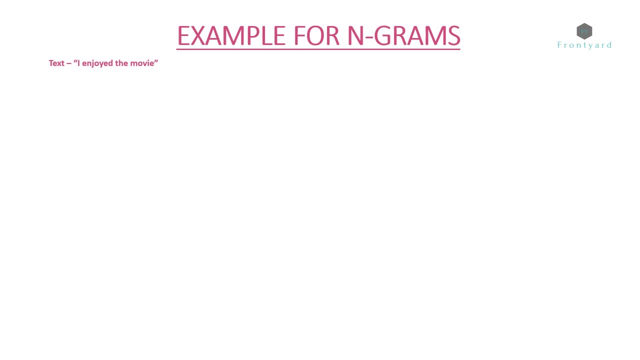 With this text, let us see how pair of words are created using N-gram. When N-gram equal to 1, the text will be considered as individual words, And when N-gram equal to 2, the text will be considered as individual words. 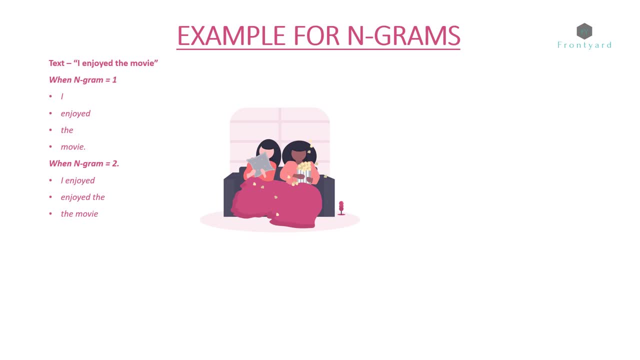 And when N-gram equal to 2, the text will be considered as individual words. The text will be considered in pair of twos: Like I enjoyed is a separate term. Enjoyed, the and the movie is two different separate terms. 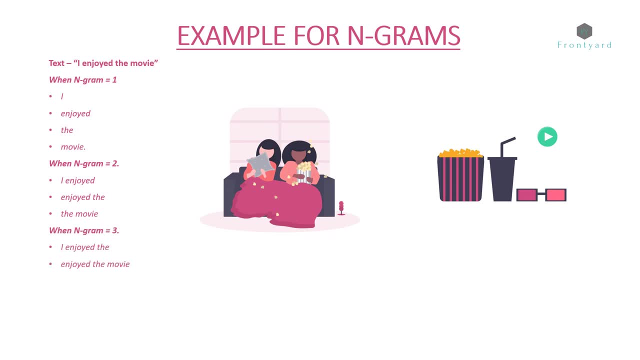 When N-gram equal to 3, the text will be considered in pair of three words. N-gram will be helpful in identifying the part of speech by using the previous word or the nearby words. POS tag, For example. when N-gram equal to 2, the 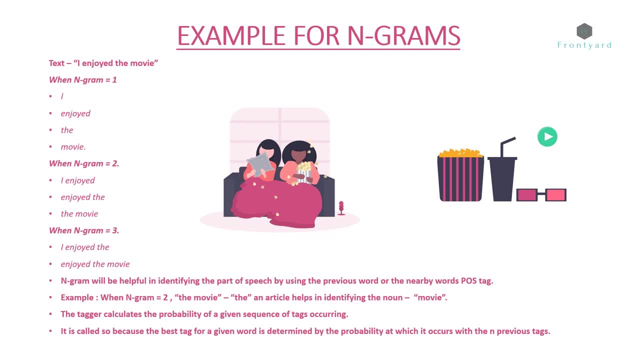 This Gi is used with the attached letter When ci talks about a movie. here, the first word is the, which is an article, and the second word is movie. This therefore occurs when N-gram equals the title in previous order. We already know that there is a rule. 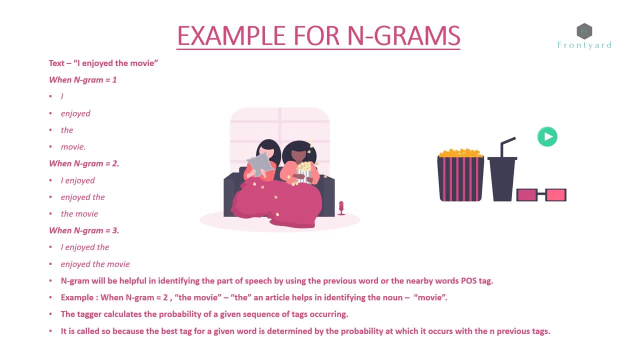 In the next level we will learn how key of this system works. that from the préf e manager figures. if i article is succeeded by another word, then it should be an N. so in this case also, it is true. So the tagger Calculates the probability of a given sequence of tag occurring. 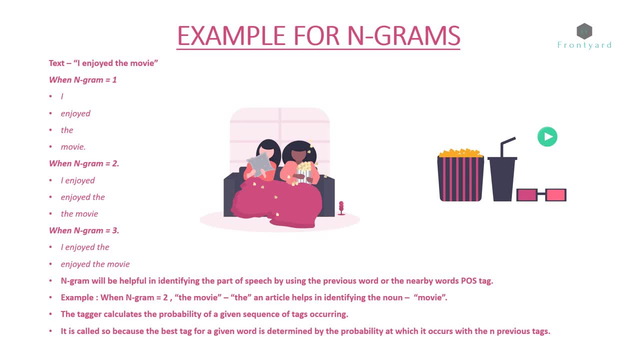 It is called so because the best tag for a given word is determining it or not. So in the next chapter we will come to know the employment of the scene and these phenomena carefully, at which it occurs with the end previous text. So here is an example for the last point. 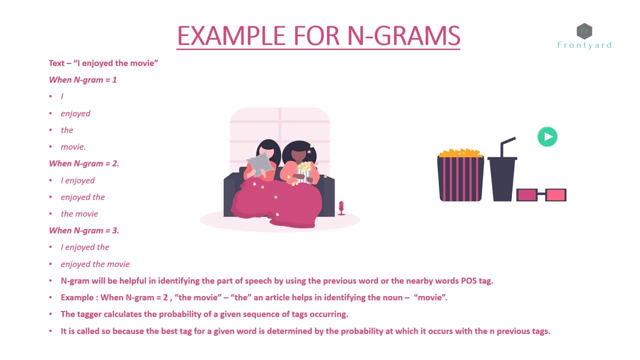 Consider the sentence I enjoy the movie and there are two more similar sentences with the movie. From this we know that movie is a noun based on the previous word, the. Now we get a new text that says movie was terrific. Now, if we see, with the previous probability of occurrences, that the past three sentences we had the term the movie in that we know that movie denotes noun. 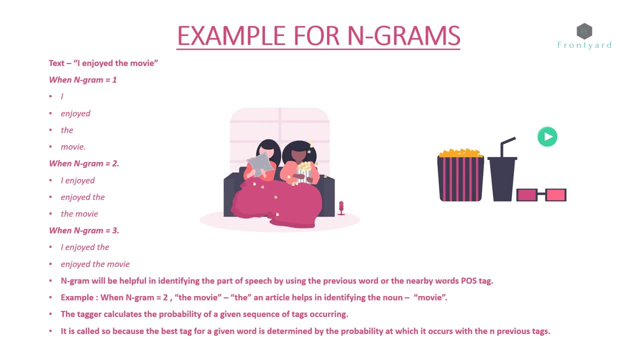 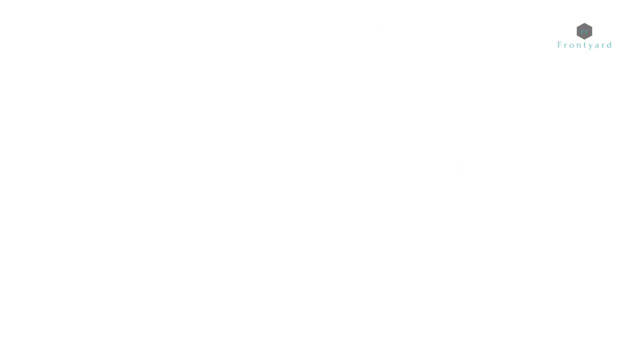 So in this sentence, when it is just movie was terrific, we will obviously know that movie denotes a noun. This is because, based on the previous sentences which we obtained and the probability which we have taken out of them, Now let us see the Python code for POS tagging. For this we need to import NLTK. 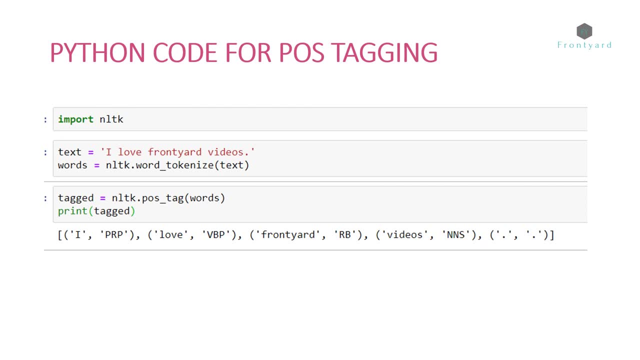 NLTK stands for Natural Language Toolkit. It is the toolkit available in Python and it is most commonly used for NLP process. The texture I am going to use is: I love Frontier Tweediers. Now we need to convert the sentence into individual words. for that we will be using word underscore, tokenize, function and.